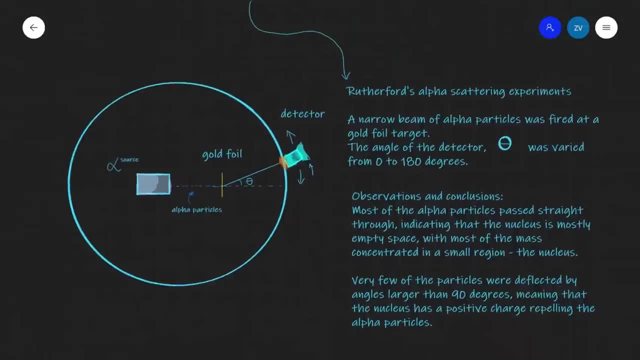 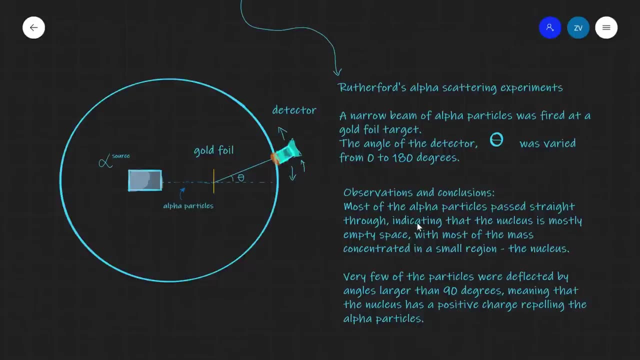 Now, what did Waterford observe? First off, he noted that most of the alpha particles were passed straight through the gold foil and this indicated the nucleus is mostly empty space, which means that most of the particles are not empty. So this indicates that the nucleus is mostly empty space, which 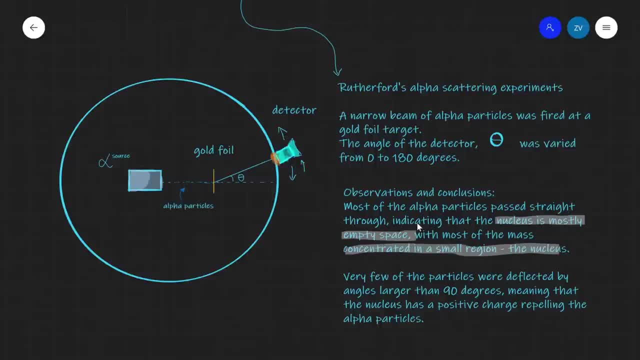 means that most of the mass concentrated in a small region, aka the nucleus. Note that very few of the particles were deflected by angles larger than 90 degrees, and this means the nucleus must have a positive charge repelling the alpha particles. If you would like to have a. 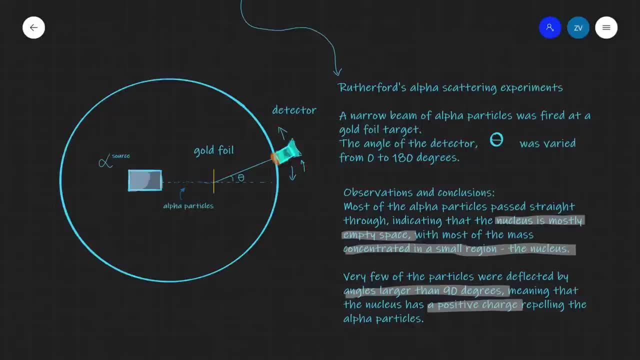 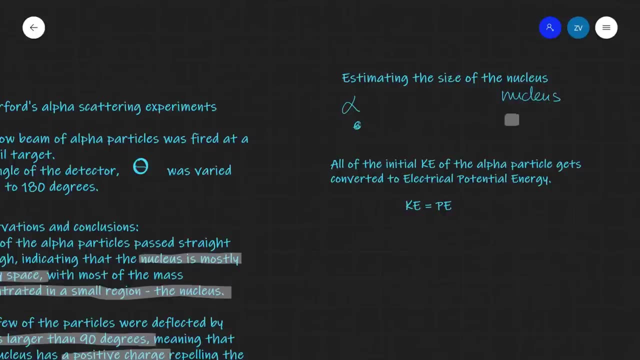 look at a detailed video of this with some animations. have a look at my video on this topic. I'll provide a link in the description of this video. Now let's estimate the size of the nucleus. Imagine that we have an alpha particle which is approaching the nucleus and at some point 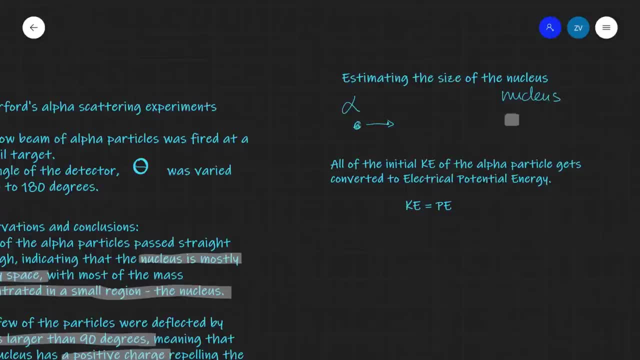 which is going to be the distance of closest approach. the alpha particle is going to have a speed of zero. So this alpha particle is going to come here, it's going to come here, it's going to come here and, aha, once it's here, it will start moving backwards. We could use this distance over. 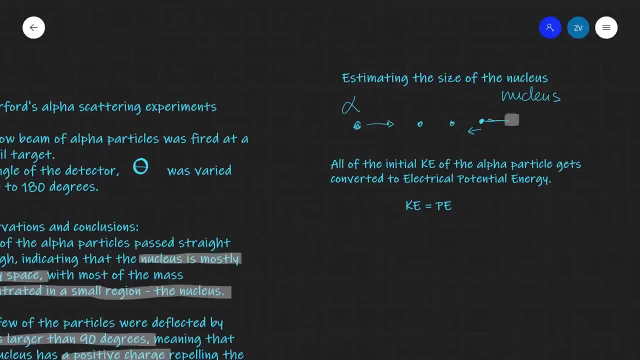 here essentially to try and get an estimate of the size of the nucleus Right. at that point all of the kinetic energy of the particle gets converted to electrical potential energy. Now Rutherford used particles which were about 7.7 mega electron volts, which essentially, if we multiply, 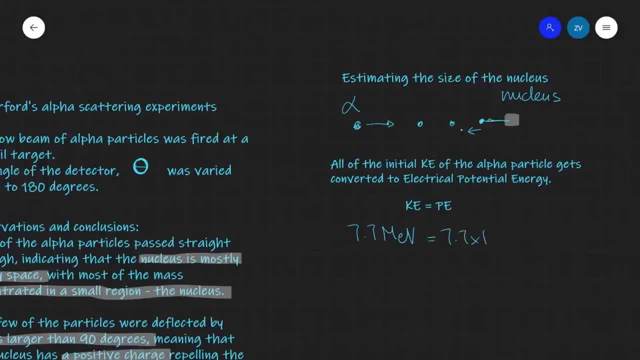 by 10 to the power of six. so let's do that: times 10 to the power of six times the electron charge. remember, if I can see the E, I multiply by it. so times 1.6 times 10 to the power minus 19,. and this: 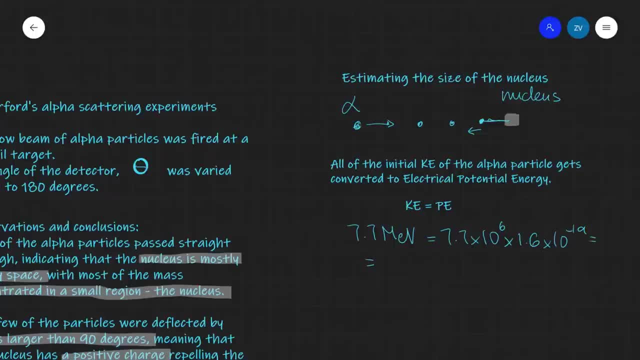 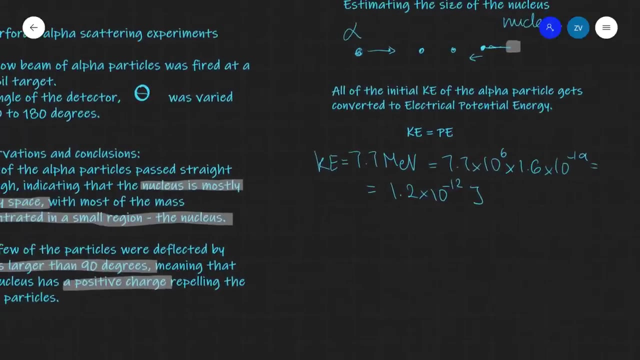 is going to give us some kinetic energy equal to approximately 1.2 times 10, to the power of minus 12 joules. So this is our initial kinetic energy. Now all of this is going to get converted to electrical potential energy, so let's do that. Our kinetic energy will be equal to 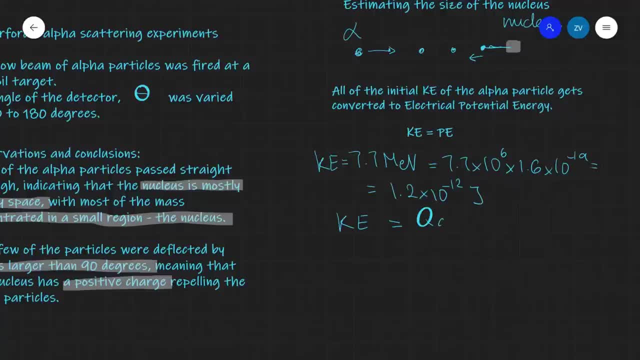 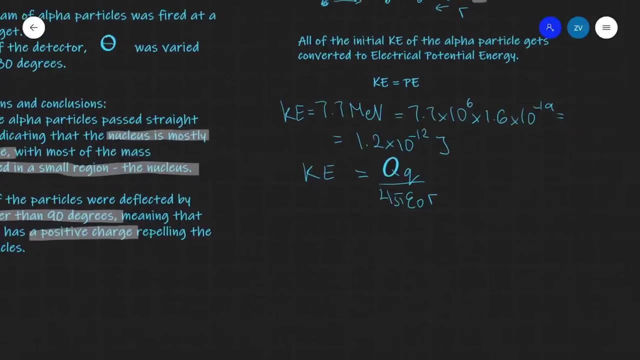 our electrical potential energy. The formula for potential energy is QQ over 4 pi. epsilon naught times R, not R squared. where R is this distance over here? Now, all we need to do, essentially, is just rearrange for R. so let's do. 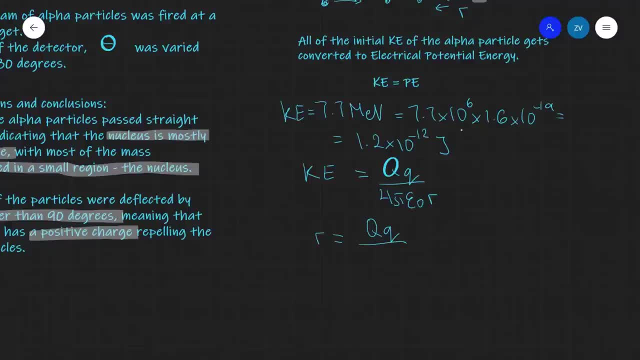 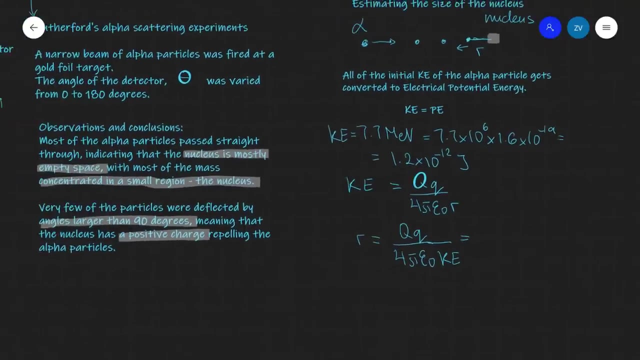 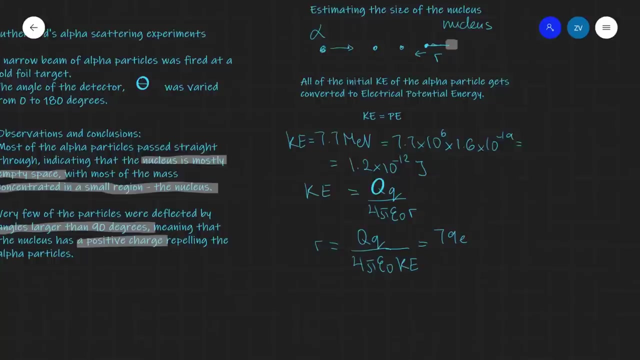 this R will be equal to QQ, over 4 pi, epsilon naught and our kinetic energy will be down here. Our charge for one of the Q's will be 79 E because we were using gold nuclei. In fact, even better, let's just draw this in yellow, indicating that these are indeed gold nuclei. 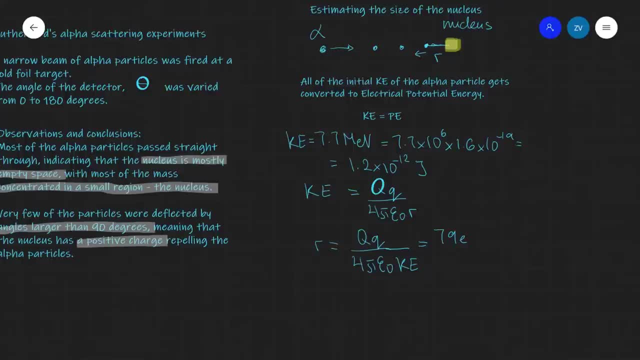 Our other charge was an alpha particle which consists of two protons and two neutrons. so this will be equal to 2 times E, where E is the elementary charge. Here Y is equal to a …. so we're going to be dividing that by 4 pi epsilon- naught times our kinetic energy. 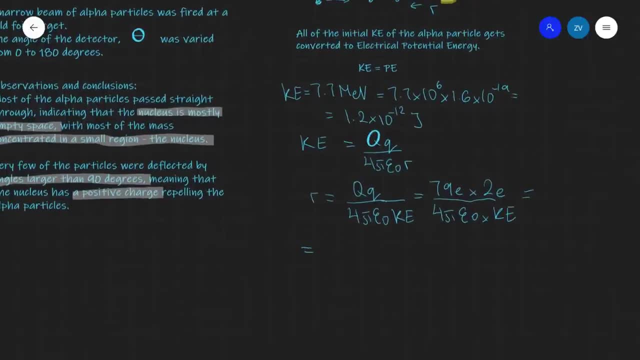 Okay, well, let's plug in some numbers now into this equation. so it would be 79 Ü times 2 times E squared. so that's going to be times 1.6 times 10 to the power of minus 19 squared. I've squared this because obviously I have two factors of E. one: 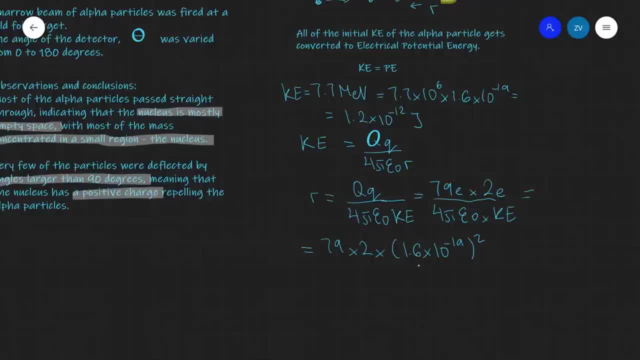 here and one here. so E times E is E squared, which is 1.6 times 10 to the power of minus 19 squared. Now I'm going to be dividing this by 4 pi times epsilon naught, which is 8.85 times 10 to the power of minus 12, multiplied by the kinetic energy which 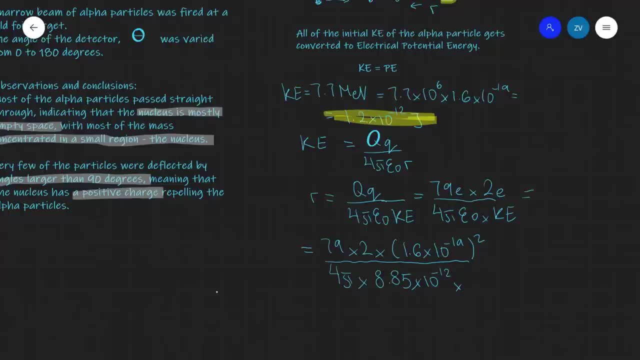 we have just up here already calculated 1.2 times 10 to the power of minus 12.. So let's write this in here: 1.2 times 10 to the power of minus 12, and if we were to plug, 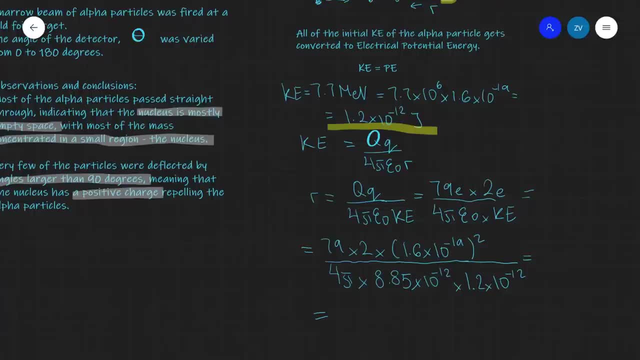 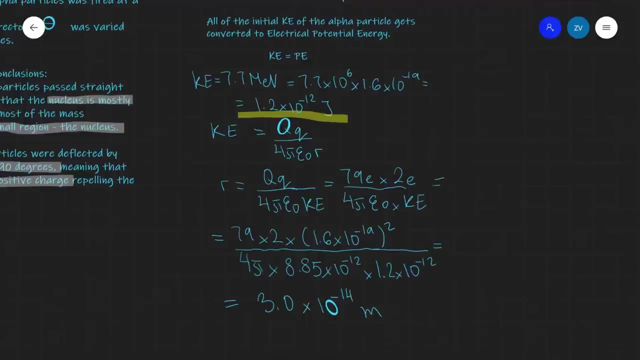 this into a calculator. let's say up to two significant figures. we're going to get approximately 3.0 times 10 to the power of minus 14 meters. So a really good estimate for the size of the nucleus is about 10 to the power of minus 14, maybe 10 to the power of minus 15 meters, And this 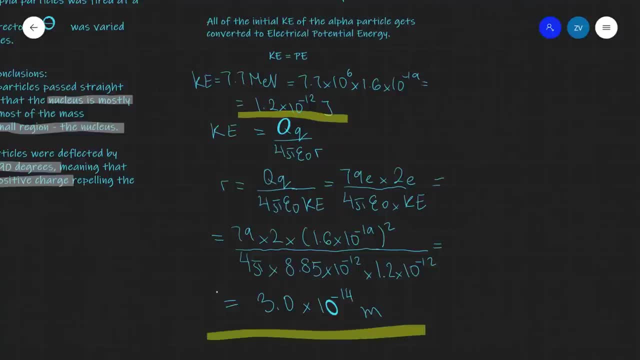 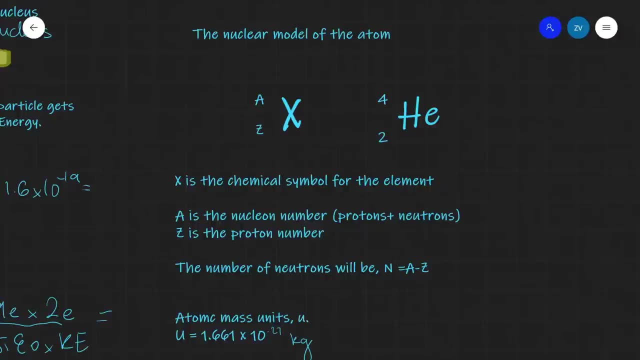 is how we estimate the size of the nucleus. Now, what's actually inside of a nucleus? Let's have a look at the nuclear model of the atom. The modern model of the atom consists of essentially x, where x is the chemical symbol for the 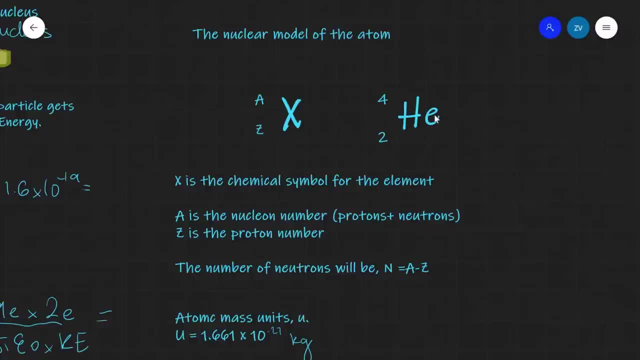 element. For instance, you could have helium, the nucleus of helium, which is represented by the atom. It's represented by this symbol. The number A in the upper left corner is the nucleon number, In other words, the total number of protons and neutrons, For instance. helium has a total of four nucleons, two protons and two neutrons. Z is the proton number and that's located in the lower left hand corner, For instance. helium is element number two, so it's going to have two protons. The number of neutrons can: 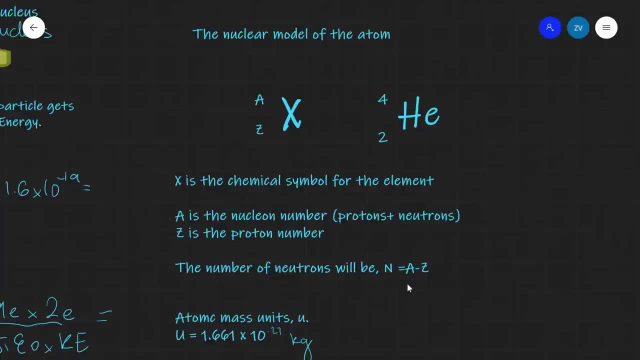 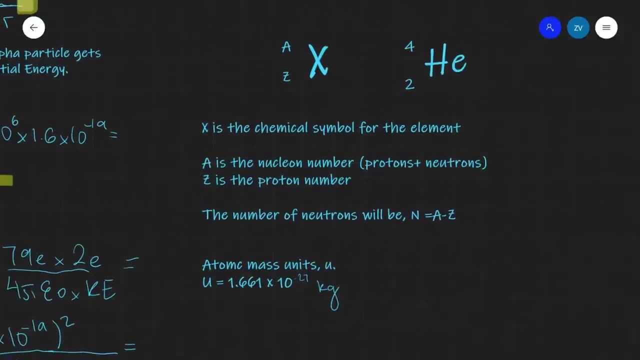 be very easily worked out using the following rule that N is equal to A minus Z. Just a little bit of revision. keep in mind that you might come across the atomic mass unit, U, which in all A-level physics exams. this constant is in your. 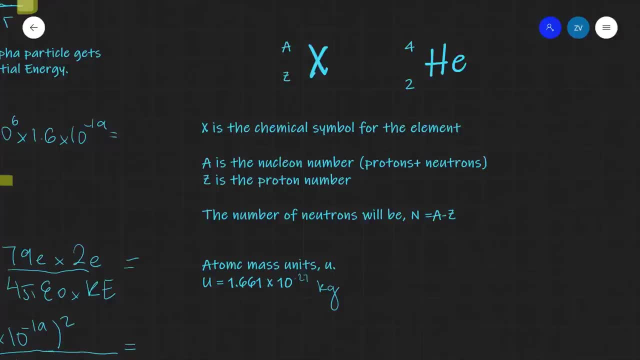 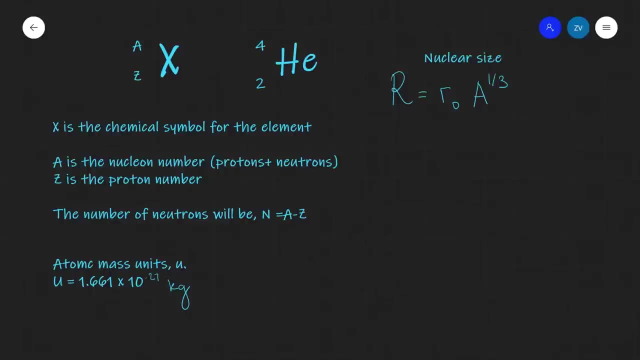 formula booklet so you don't need to remember it, but it's about 1.661 times 10 to the power of minus 27 kilograms. The nuclear size is given by the following equation: R is equal to R naught A to the power of a third. This makes: 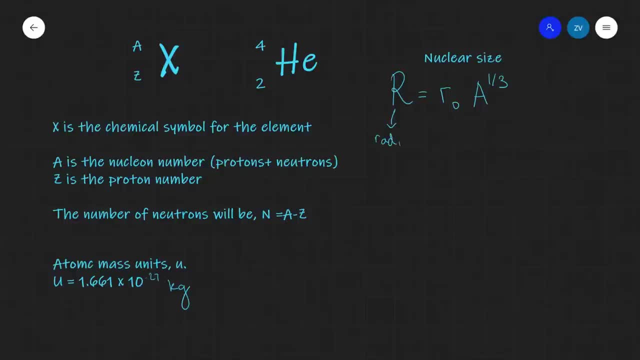 sense. So R here in this equation is the radius of the nucleus. R naught is a constant. it's approximately 1.2 femtometers. Remember femto is 10 to the power minus 15, so this really is about 1.2 times 10 to the power of minus 15. 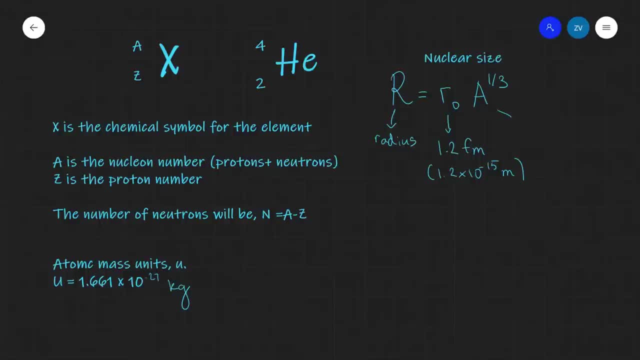 meters, and A, of course, is your nucleon number. So this makes sense essentially: the larger your nucleon number is, the larger the radius is. When A is equal to 1, your equation becomes simply that R is equal to R0.. So you can think of this as: 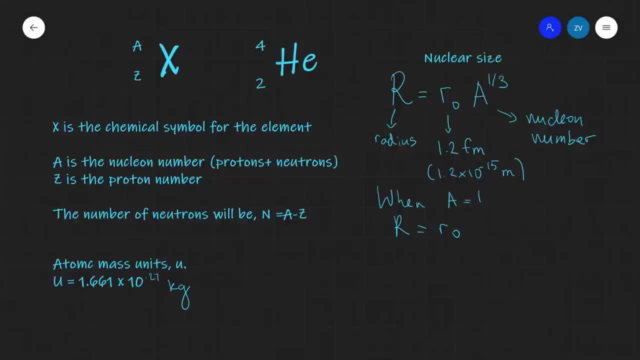 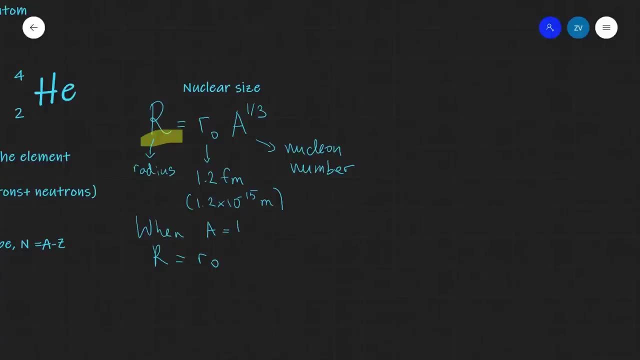 essentially this roughly the size of a hydrogen nucleus. Using the following equation, we could actually estimate the density of the nucleus. All we need to do is use the equation that density is equal to mass over volume. Now let's assume that the nucleus is a tiny sphere. If that's the case, our density will be. 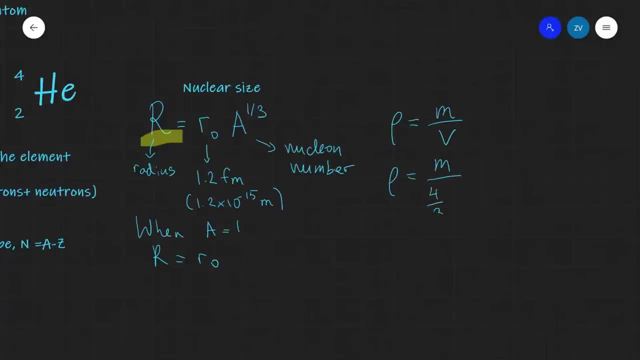 given by mass divided by 4 third pi, R cubed. However, we've already have an equation here for R. I've highlighted it over here- So we could write down that our density rho will be equal to the mass divided by 4 thirds pi times R0. A to the power of 1 over 3, all of it. 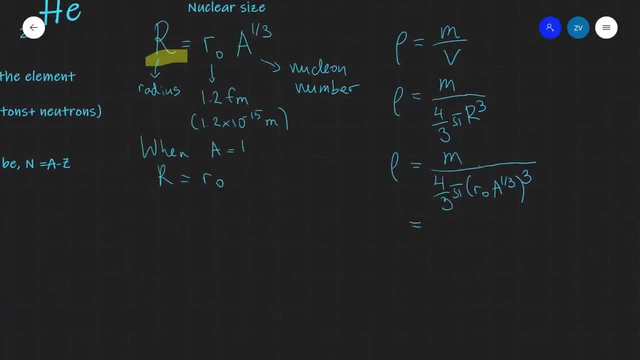 cubed. Okay. well, our density will then be equal to the mass divided by 4 thirds pi R0 cubed. And if I cube A raised to the power of 1 third, I'm just going to get A Now. using this equation, we could calculate the density of any 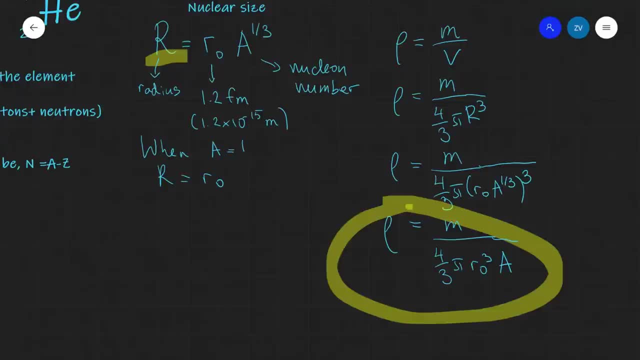 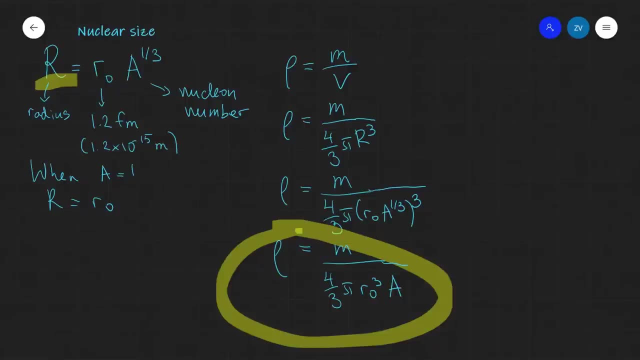 nuclear matter. Now, the density of the nucleus itself is extremely high. So most nuclei have a density of approximately 10 to the power of 70. So if we're calculating, the density is about 10 to the power of 70 kilograms per meter cubed. Remember, most of the mass of the atom is concentrated in 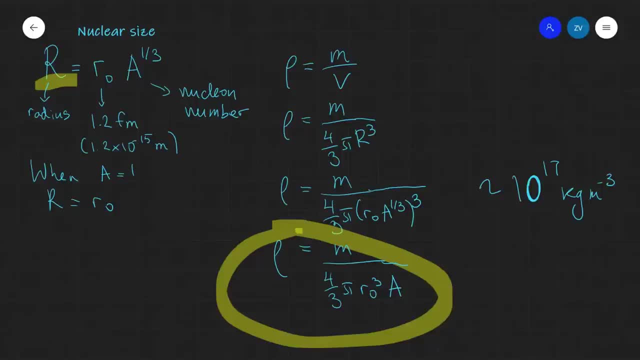 the nucleus. so the density of the atom itself is not particularly high. It's somewhere about one and a half kilograms per meter cubed. But the density of the nucleus itself is approximately 10 to the power of 17. So something which is really worth. 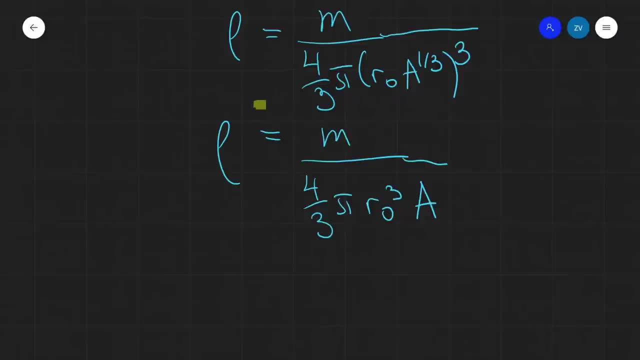 adding in the following equation: for the density of nuclear matter is that it seems to be independent of the nucleon number A. Why is that? Well, because our density is equal to the mass divided by the volume. you can assume essentially that your mass is proportional. let me just write this over here on the side. 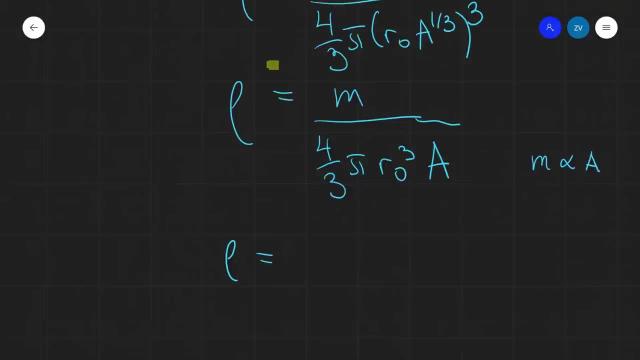 that your mass is proportional to the mass divided by the volume of the atom. This is because the mass of a proton is approximately the same as the mass of a neutron. Of course they do differ by a few parts in 10, to the power of minus 27. but 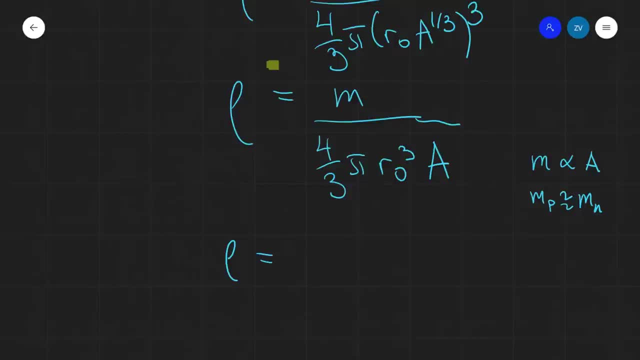 they're very, very similar. Because of that, the overall mass will be a multiple of, essentially, the mass of the individual nucleons. So you can think of the mass of the nucleus as proportional to the nucleon number. In other words, let's call that Ka for some. 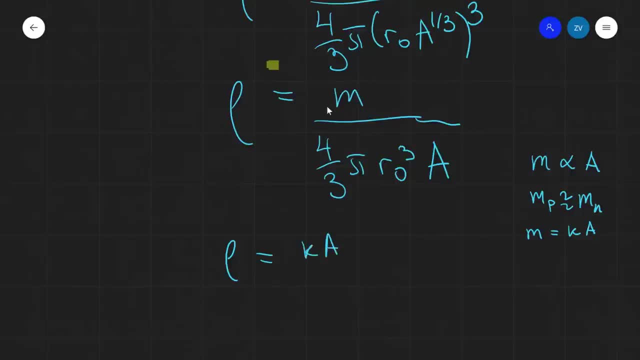 constant K, Our nuclear density will be Ka, over 4 thirds pi, r0 cubed times A. And notice, we can do my favourite thing in physics, which is to cancel terms out. and our nuclear density is independent of the nucleon number, So the mass of the atom is equal to the mass divided by the volume you can assume. essentially, 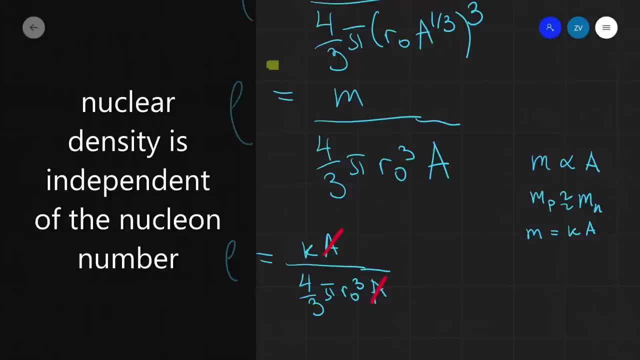 that your mass is proportional to the mass of the atom. So you can think of the mass of the nucleon number. So this means that the hydrogen nucleus is going to have approximately the same density as the uranium nucleus, which is going to have approximately the same density. 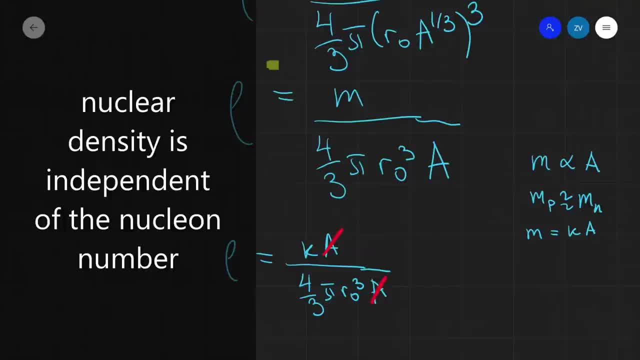 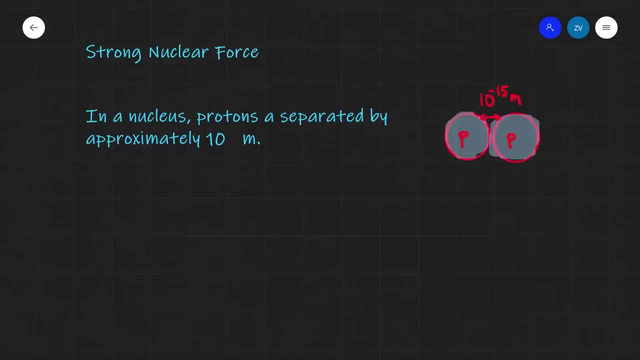 as the carbon nucleus. This also tells us that the individual protons and neutrons inside probably have a very, very similar spacing between them, regardless of which nucleus we are talking about. So let's have a deep look inside of the nucleus. Let's imagine that we have something like helium, for instance, where we have two protons. 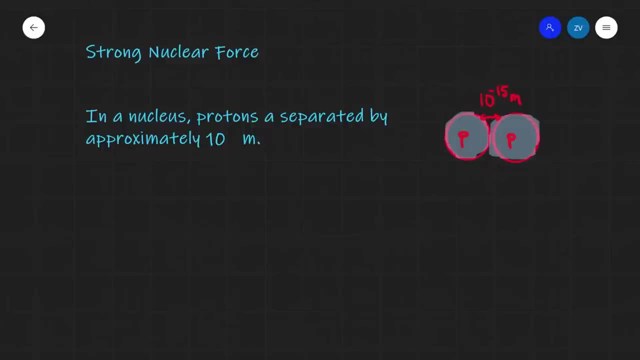 The distance between the individual protons and their nucleus is of the order of 10 to the power of minus 15 meters. Because the protons are of the same charge, this means that they will experience an electrostatic repulsive force. We can calculate that force. 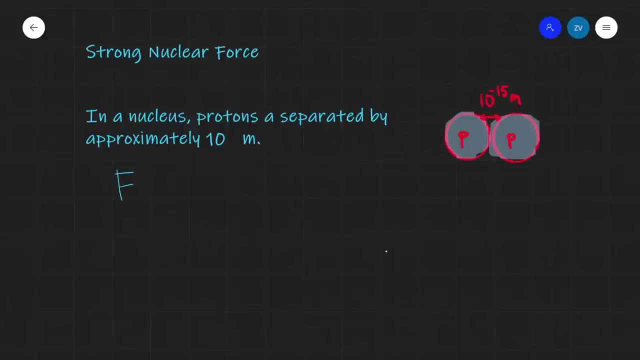 using Coulomb's law. Remember. Coulomb's law says that the force is equal to Q, Q whole over 4 pi. epsilon naught r squared q is just the elementary charge, so in this case that'll be q times q, so it's going to be 1.6 times 10 to the power of minus 19. all of it squared, and now we're. 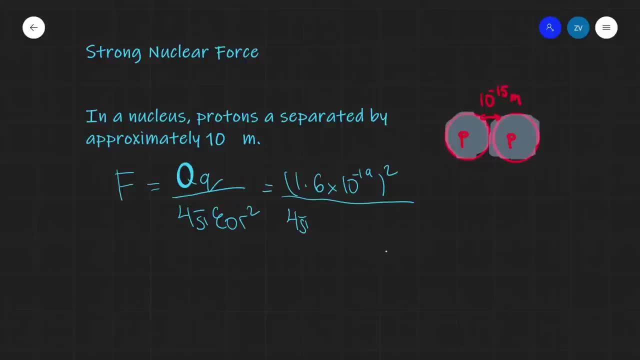 going to be. dividing this by 4, pi, epsilon naught is 8.85 times 10 to the power of minus 12, and our distance is tiny, so that's times 10 to the power of minus 15 squared. putting this into a calculator: 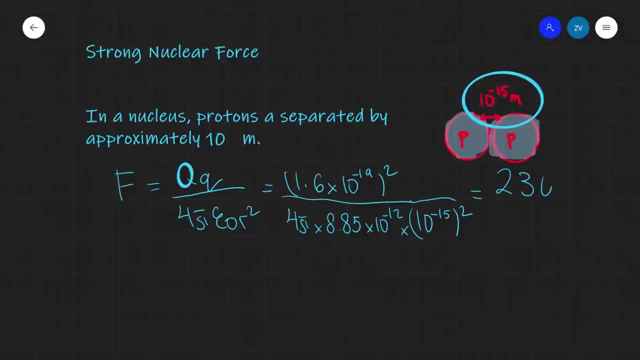 we are going to get approximately 230 newtons. now. this is an absolutely huge force which is being applied to two subatomic particles. so there's a force of 230 newtons acting on something of a mass of approximately 1.6 times 10 to the power of minus 27, which would 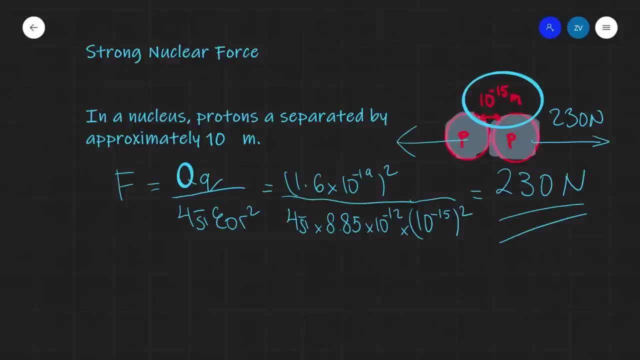 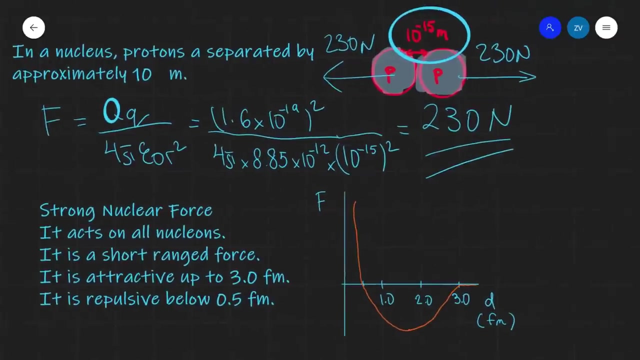 which would essentially create an enormous acceleration. and if this electrostatic propulsion was the only force acting, all of matter should just essentially separate and very quickly accelerate to the speed of light. luckily that's not the case. let's have a look at the properties of the strong nuclear force. the very fact that matter exists means that there has 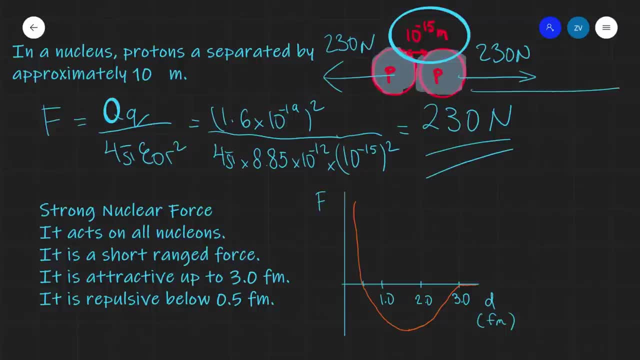 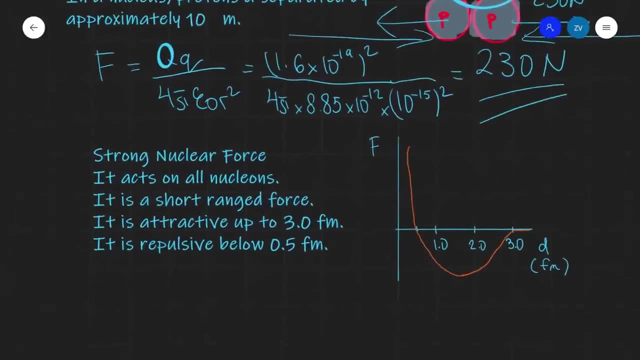 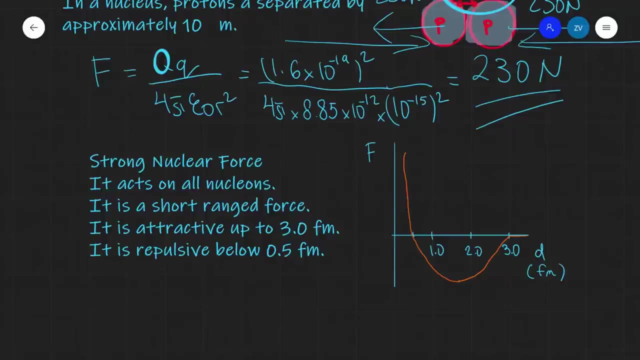 to be a much stronger force which is opposing that. you coulomb repulsion and it's keeping the nucleus together. here comes the strong nuclear force. cool facts: it acts on all nucleons, so that's protons and neutrons. it is a short range force. 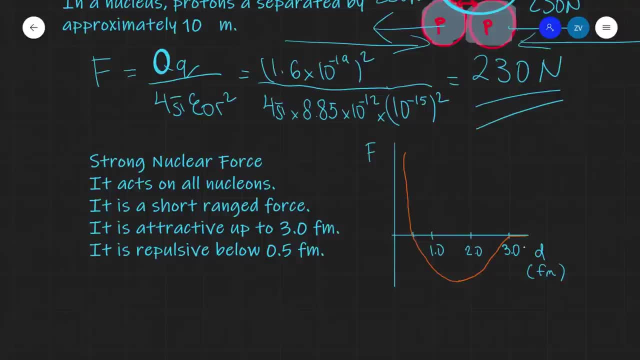 we can see how, above three femtometers on this graph, the force is essentially zero. it is attractive up to three femtometers and is repulsive below higher half a femtometer. in other words, in this region over here from 0.5 to approximately three femtometers. 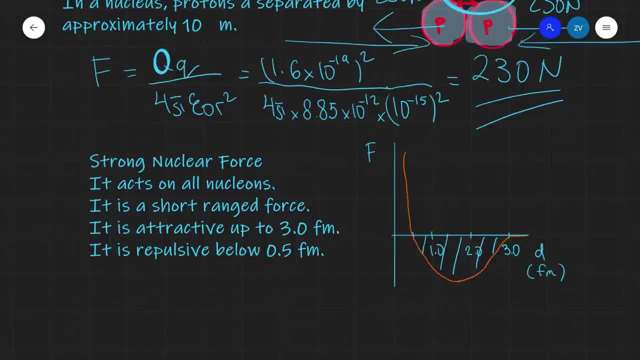 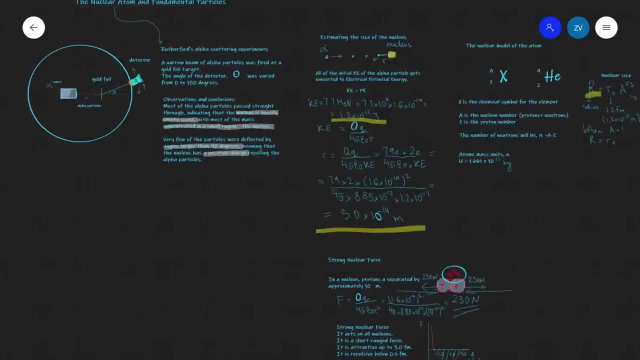 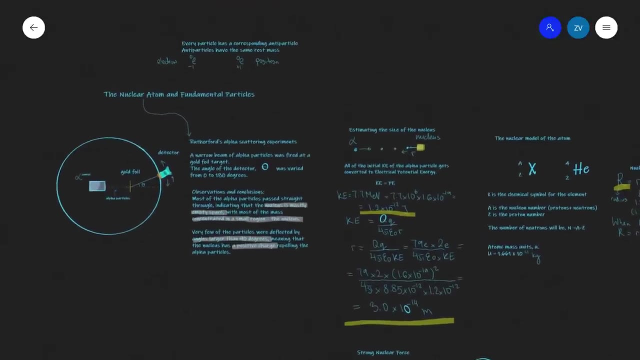 the force is attractive and it is very, very strong, keeping the protons inside the nucleus together. so so far we have revised quite a lot about the nuclear atom. let's have a look at fundamental particles as well. the first aspect that we're going to revise are the nuclear atoms and the 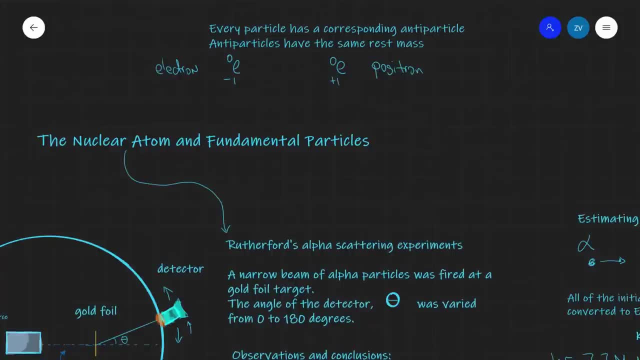 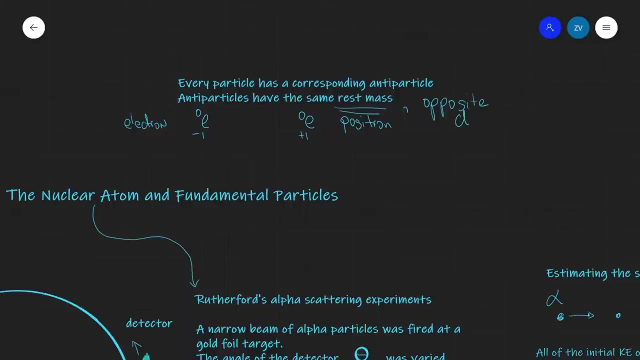 particles are antiparticles, so every particle has a corresponding antiparticle. antiparticles have the same rest mass, and this is really important. however, they do have the opposite charge. for instance, we have an electron, which, of course, is negative. however, its antiparticle is known as the positron. 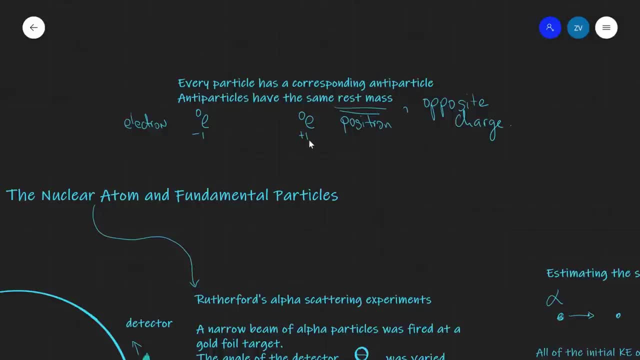 which has the same charge but with opposite signs. so we have an antiparticle which is negative. and So, whereas the electron has a charge of minus 1.6 times 10 to the power of minus 19 coulombs, the positron is going to have a charge of plus 1.6 times 10 to the power of minus 19 coulombs. 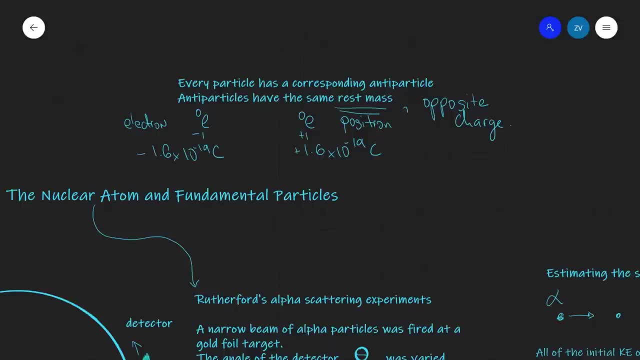 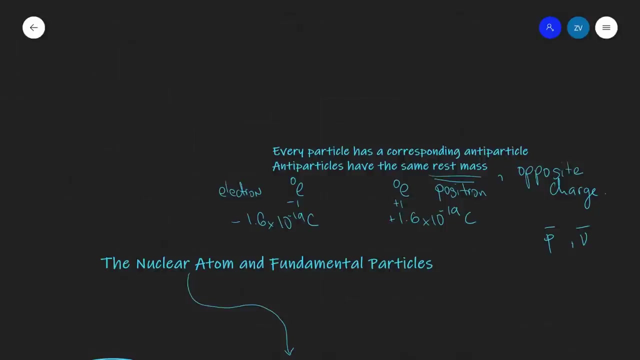 Typically we tend to essentially write down antiparticles with a little dash on top. For instance, this over here would be an antiproton, this over here would be an antineutrino. So talking about fundamental particles and antimatter and essentially fundamental physics. 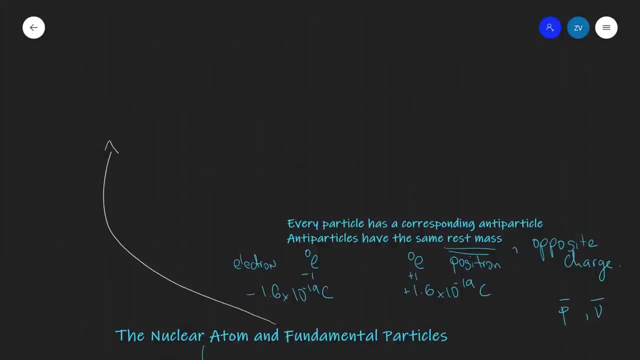 we need to mention the four fundamental forces, or also known as the four fundamental interactions. Probably the first one which we've studied is the gravitational force. So let's just write, Let's write down here forces which are fundamental. So the gravitational one is one of them. 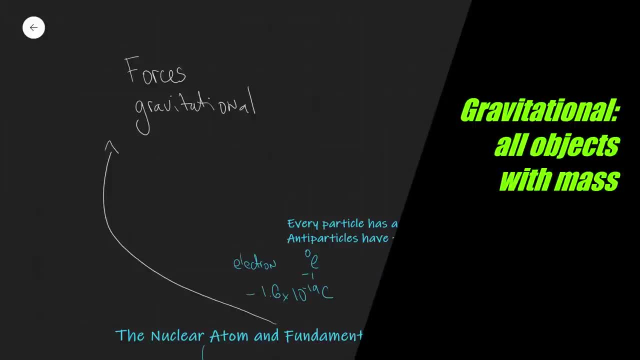 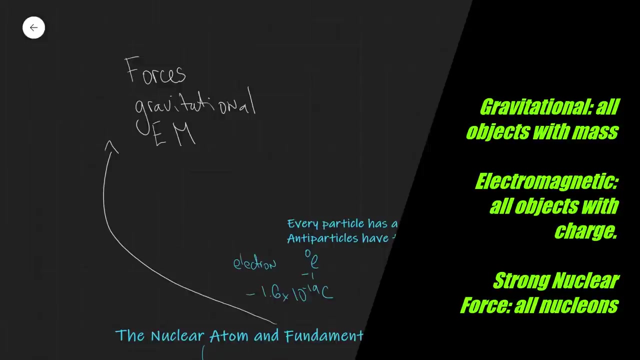 And this is experienced by all particles which have mass. The other fundamental interaction or fundamental force that we have studied is the electromagnetism or the electromagnetic interaction, And this is experienced by all particles which have charge. We've also included the strong nuclear force. 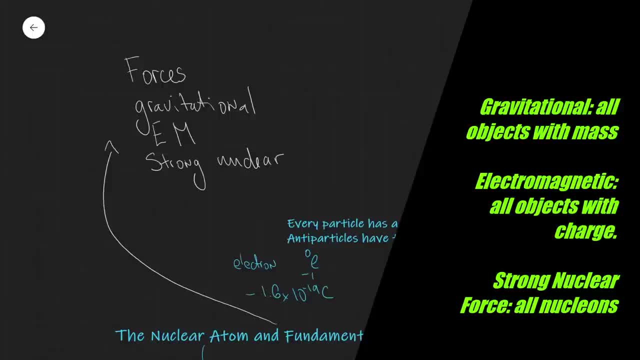 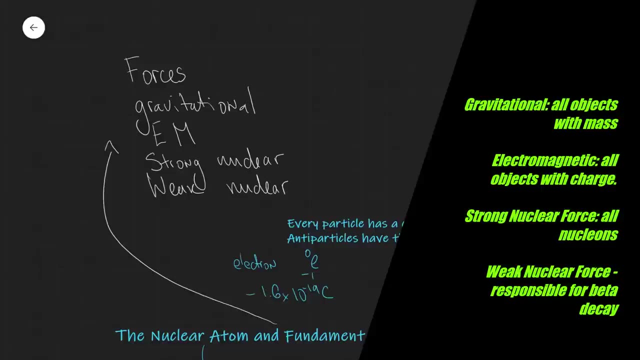 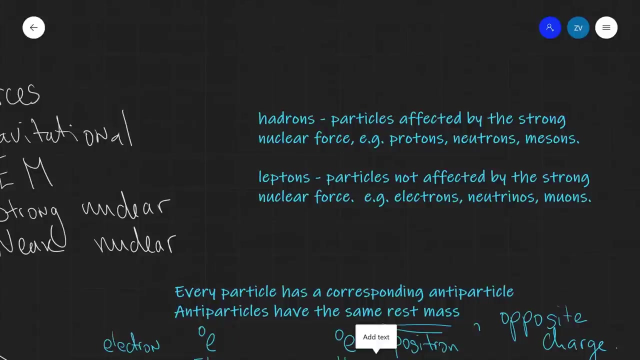 And the strong nuclear force is experienced by all nucleons. So the strong nuclear force is experienced by all nucleons. We also have the weak nuclear force which is responsible for beta plus and beta minus decay. We can split the subatomic particles into two main classes. 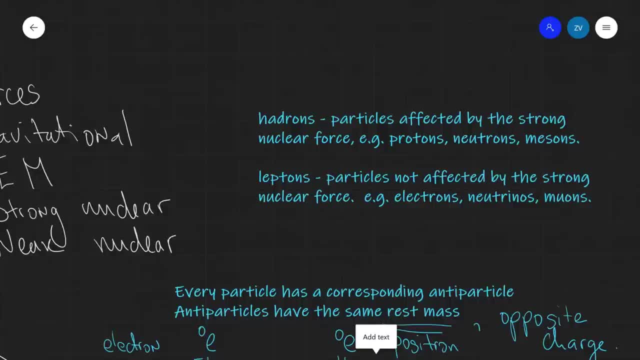 One of them is hadrons. For instance, we have the large hadron collider, which collides hadrons. These are particles which are affected by the strong nuclear force. Examples include protons, neutrons and a new class of particles called mesons. 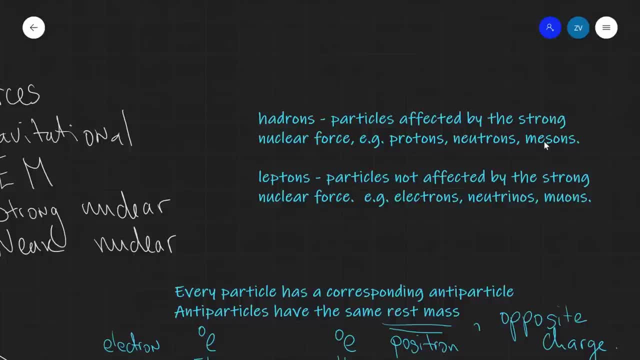 which we have not talked about yet, but they basically consist of a quark and an anti-quark. The other class of particles, called leptons, are particles which are not affected by the strong nuclear force. Examples include electrons, neutrinos and muons. So what are protons and neutrons? 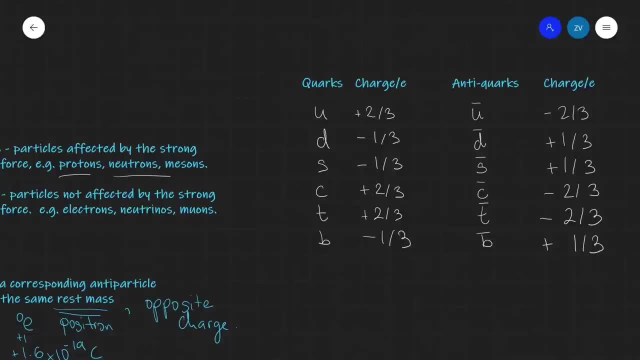 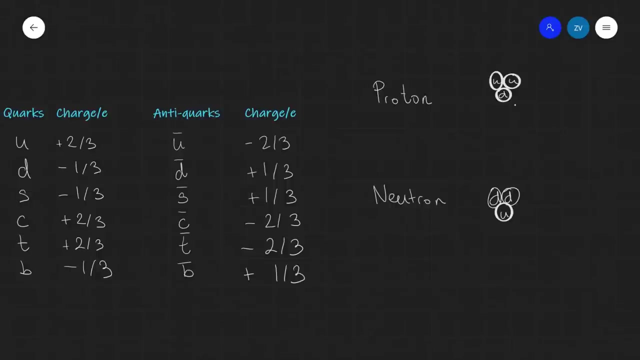 actually made of Well. protons and neutrons are not fundamental particles, Mesons as well, they're not fundamental. They're all made out of quarks. So a proton, for instance, consists of two up quarks and a down quark and a neutral. 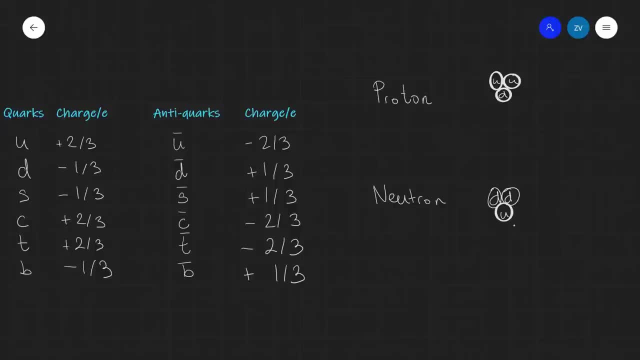 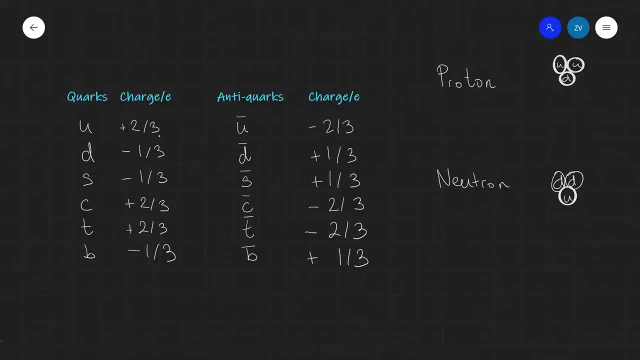 consists of two down quarks and an up quark. The quarks have a fractional charge, so in terms of E, an up quark is plus two-thirds, a down quark is minus a third. These values for the quarks and the corresponding anti-quarks are given. 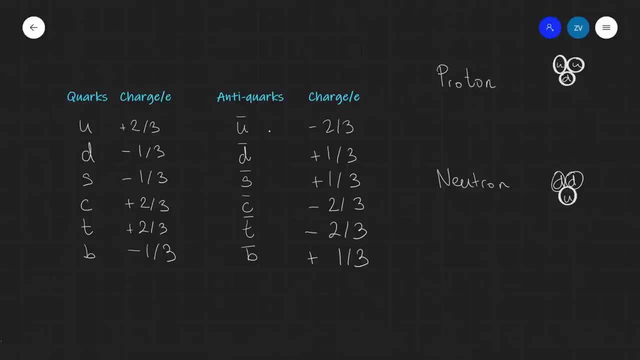 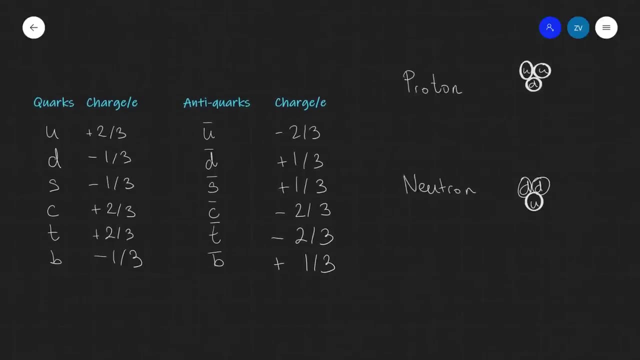 in your formula booklet. We could use them to work out the following equations. Let's say the charge of a proton. For instance, a proton consists of two U's and a D, which would mean that the overall charge for a proton will be equal to plus two-thirds E. 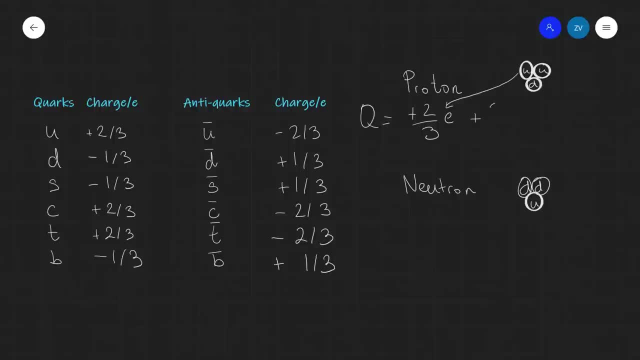 So that's the charge of one of the up quarks, plus two-thirds E, which is the charge of the other up quark. And then we also have a down quark which has a charge of minus a third E. So this over here is the charge of the down quark. So plus two-thirds, plus two-thirds. 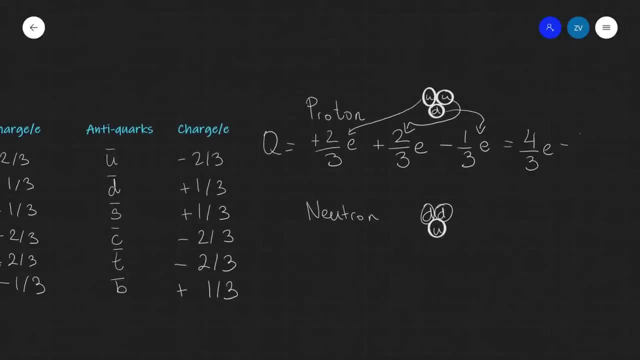 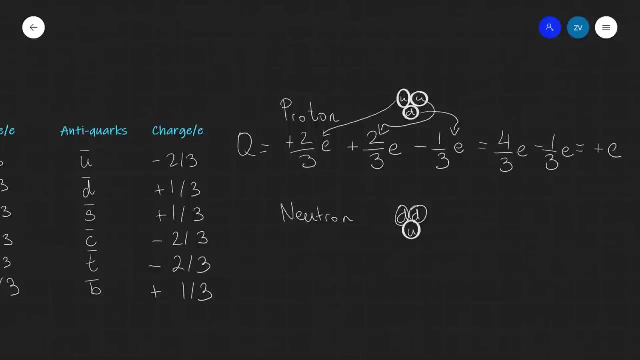 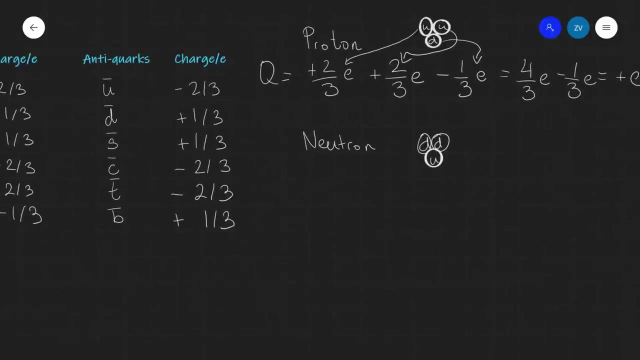 is going to give us four-thirds E minus a third E, which of course is going to give us three over three, which is just plus E, and that's the charge of a proton. A neutron, on the other hand, consists of two D's and a U, and we can see over here that the charge of a proton is going to be. 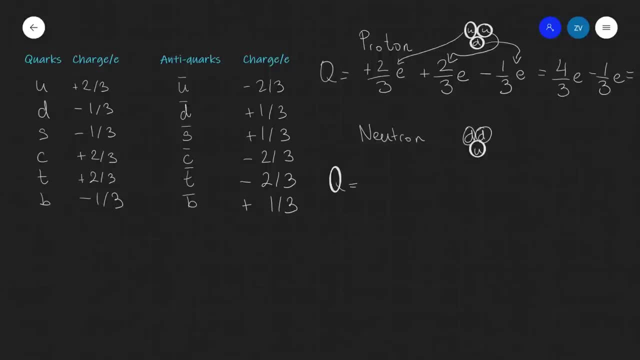 equal to minus two-thirds E. So that's the charge of one down quark. The other down quark also has a charge of minus third E, and a up quark has a charge of plus two-thirds E Minus a third. 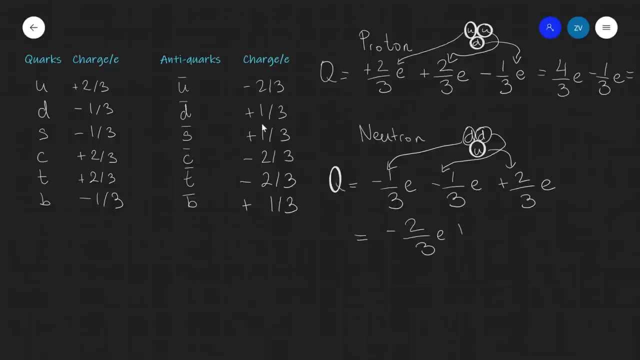 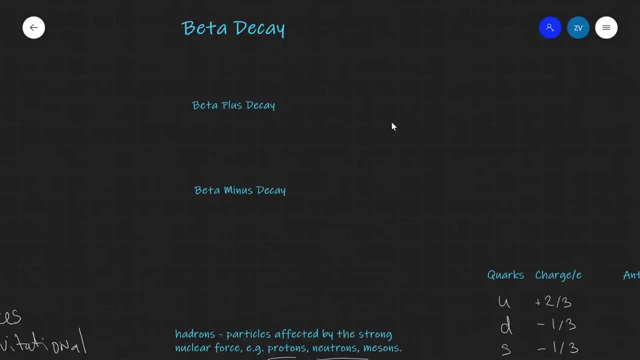 minus a third is minus two-thirds E plus two-thirds E, And we can see that the neutron is going to have an overall charge of zero. Now the final aspect which we're going to be looking at today is beta decay. There are two types of beta decay: beta plus decay, and 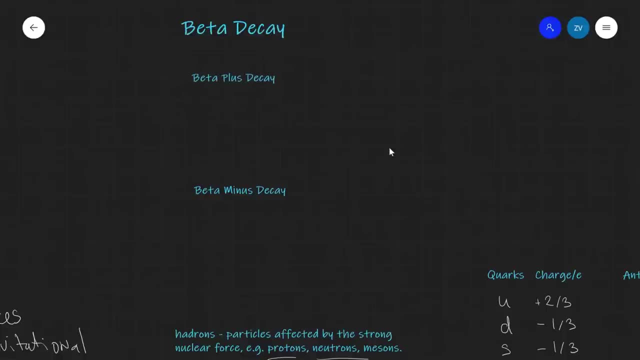 beta minus decay. Now in both of them you either have a proton turning into a neutron or a neutron turning into a proton. In beta plus decay we actually have a proton which is zero, And in beta minus decay there is a proton which is going to turn into a neutron. Now let's balance out this. 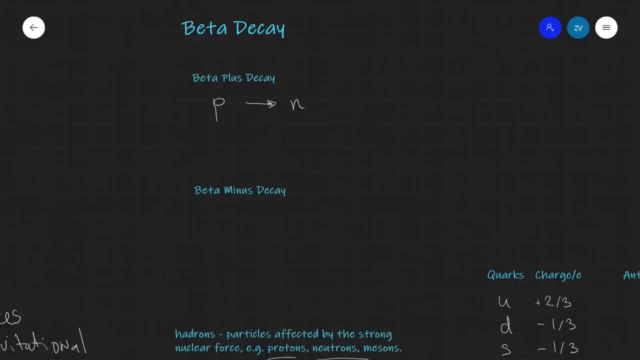 equation: A proton is going to have a proton number of one and a neutron is going to have a proton number of zero. In each case the nuclear number is going to be one. Charge is not conserved at the moment. We have a proton of charge one or plus one and a neutron of overall charge of zero. So in 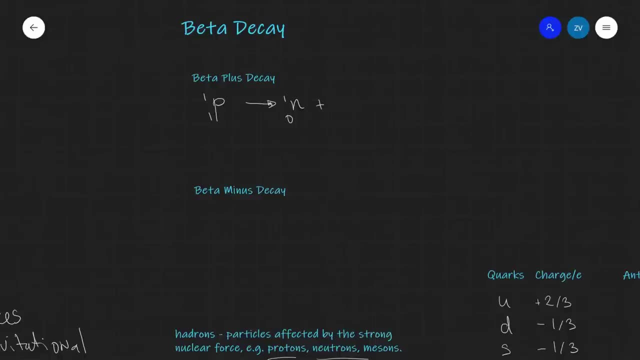 So, in order to balance out this equation, we're going to need a beta plus particle, which is a positron, So that's going to be plus one zero. We also get a little neutrino. overall, The neutrino has almost no mass and has no charge, and it's not a nucleon. 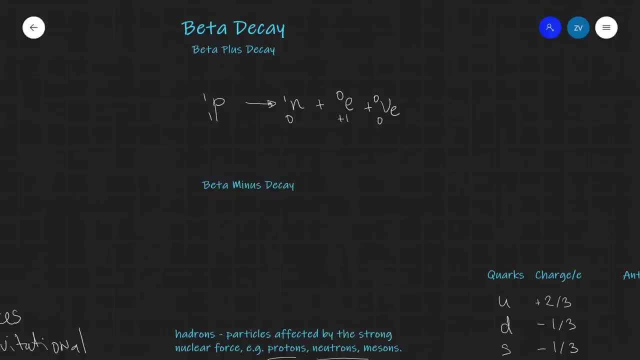 Remember the quark composition of the proton. So a proton was an up, up and down quark which is now turned into a neutron, which is a down, down and an up quark. So in this beta plus decay, what we actually have is one of those up quarks has turned into a down quark. 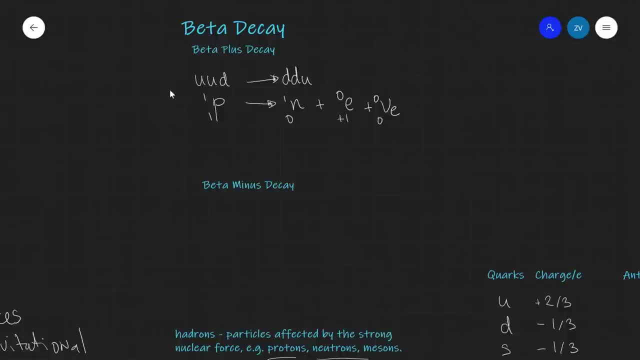 So another way of writing down the beta plus decay equation in terms of quark composition is an up quark which turns into into a down quark, plus we get a positron and a neutrino. Let's do the same for beta minus decay.